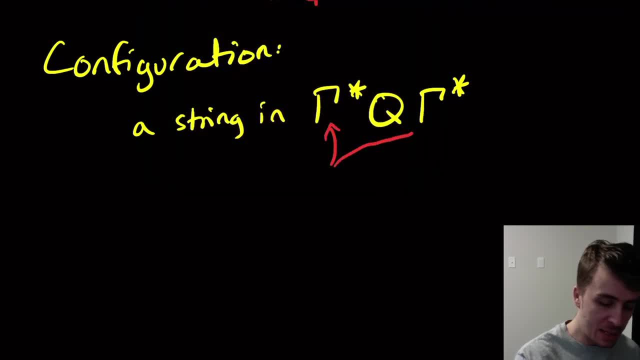 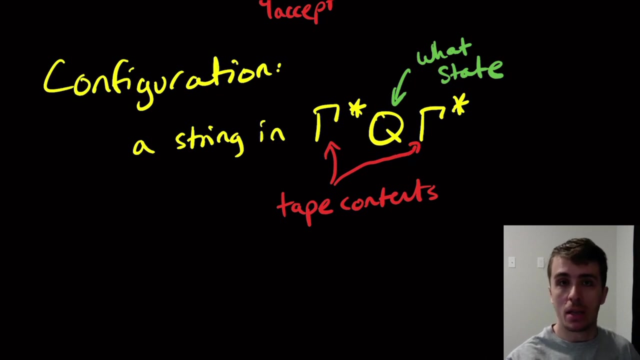 And what that means is that the two gamma stars are indicating the tape contents. the q in the center is saying what state we are currently in. And how do we actually figure out where we are on the tape? Well, the q is inserted at the right place to indicate where the tape head. 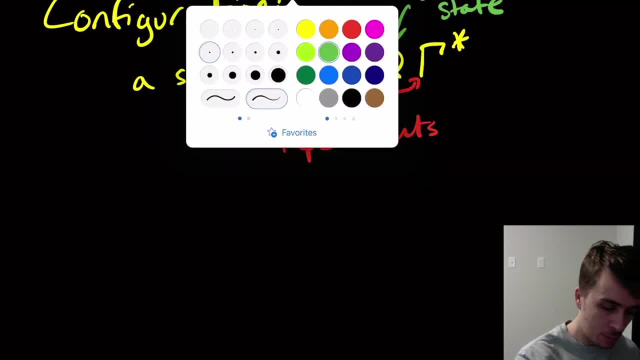 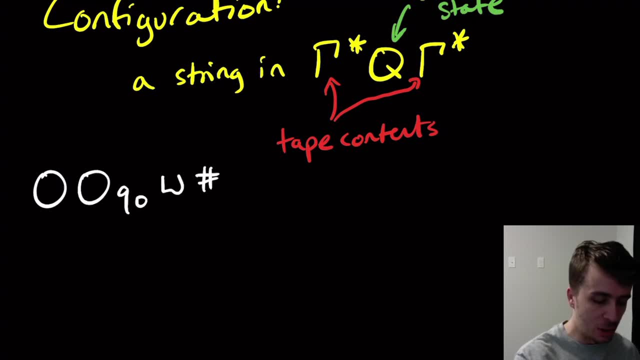 actually is. So just as an example, So if we have, say, 00q0, a blank pound sign or something, then this is saying that this is the first gamma star in the notation. So this is gamma star, right here. Or a string in gamma star, I should say This is the q or the state in this, in the set q. 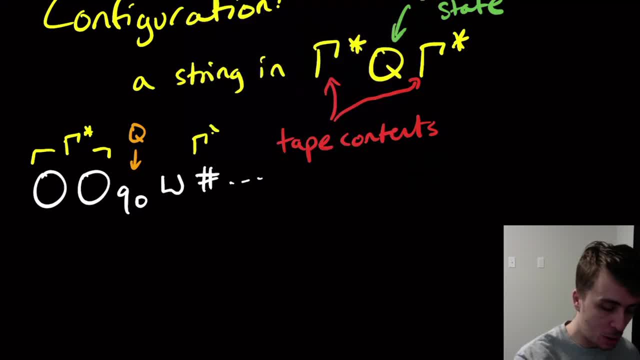 And we have the other gamma star over here. And how do we figure out what character we're looking at on the tape? Well, there are, there are two possibilities here. Either it could be the character to the left or to the right of the cell, not the cell, the character where the state is. 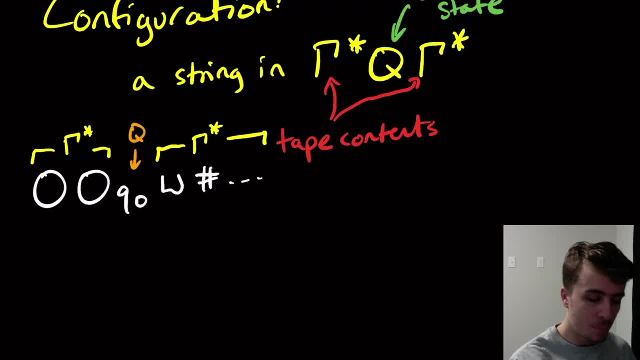 So either it's looking at this cell or it's looking at this one. The way that we're going to do it here is we're going to look at the one on the right. So we can actually notice from this that the starting configuration- I'm going to abbreviate it, config- is q0 and then w1, w2, up to 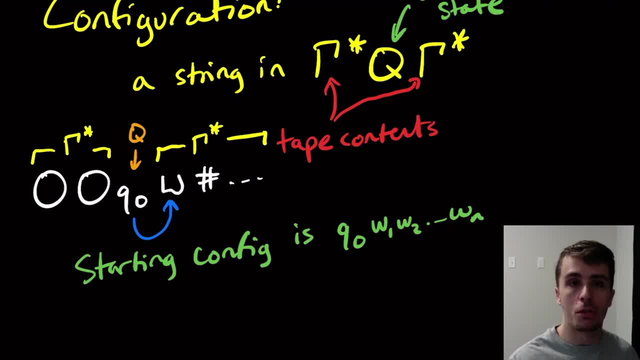 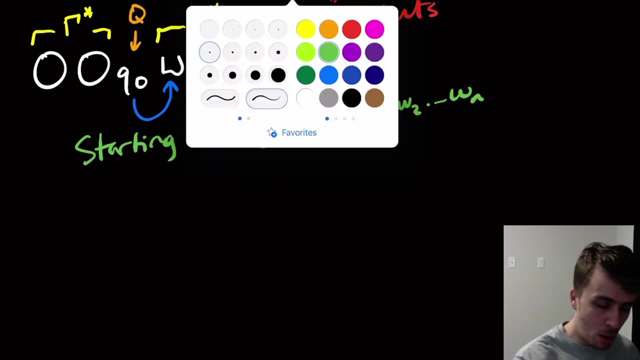 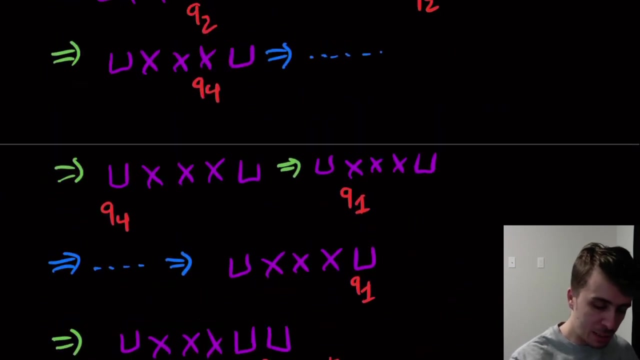 wn. So if the input string is w1 through wn and the starting state is q0, then the Turing machine must start like this: It must have the q0 first and then the input after that. Okay, so what about all of those configurations that we did earlier? And also note that I wrote the state below the 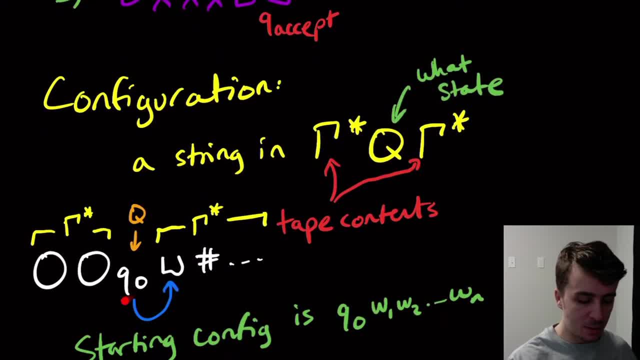 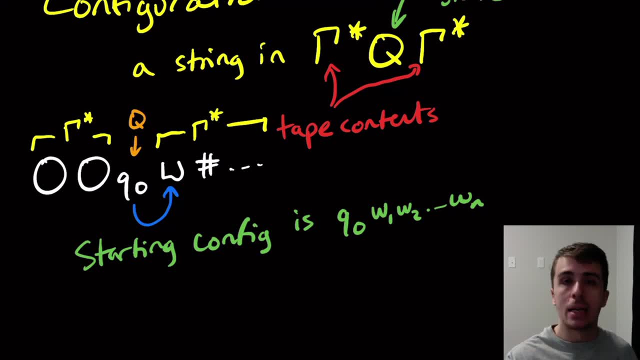 character we're looking at, and here we're writing it to the next, right next to it. We want to do it this way because we want to actually write them out as a string and so that we know a lot of things about strings, and so we want to be able to. 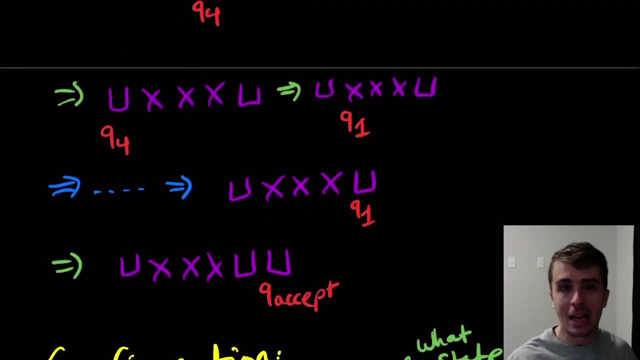 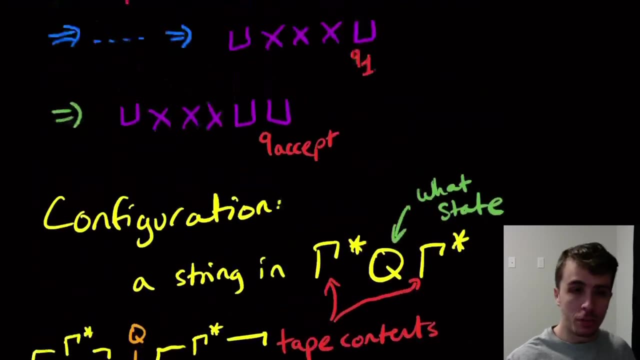 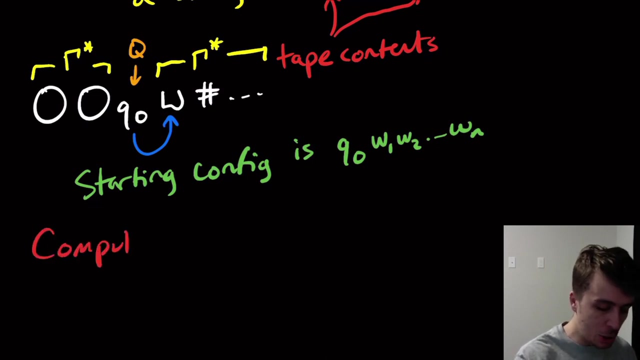 manipulate strings that way, Whereas up here these weren't actually strings, it was just a visual representation of what was going on. So we have a bunch of configurations essentially up here, and what we're going to call a computation is a sequence of configs, And what I should note here is that this is a finite sequence of configs. 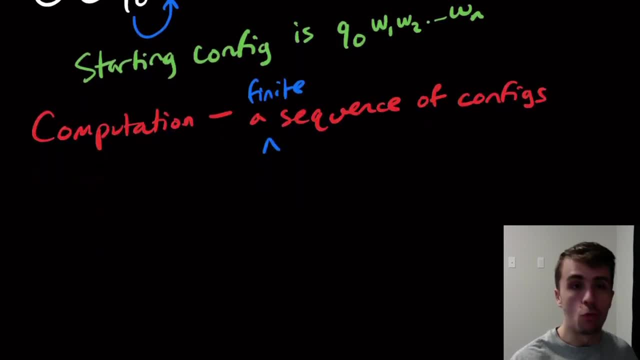 Okay. so if I have a Turing machine that runs forever, then that is not a computation right because it's not a finite sequence of configurations of that Turing machine. And then let's just call it, say c0 up to cn, let's say, Let's say that's the finite list of configurations. 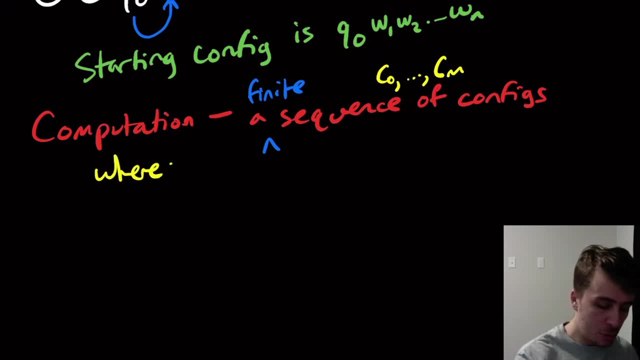 that Turing machine goes in And we have some qualifications on what those can be. So we have that c0 is the start config and ci, or I should say i plus one, comes from c, sub i from one transition. So if we apply a transition from ci, we get ci plus one. 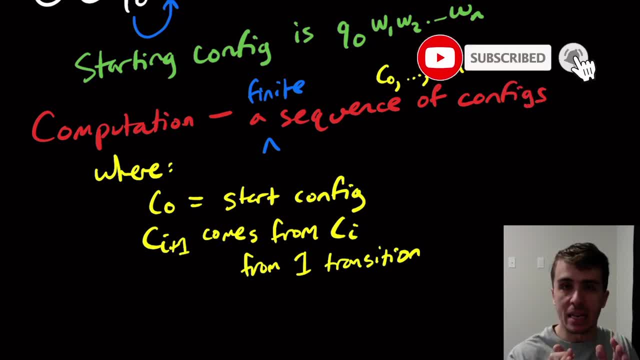 And this is. there's only one sequence of configs, assuming it's a finite sequence. There's only one possible sequence because the Turing machine is deterministic. There's no possible choice that is ever going to happen here. Okay, what does comes from mean. 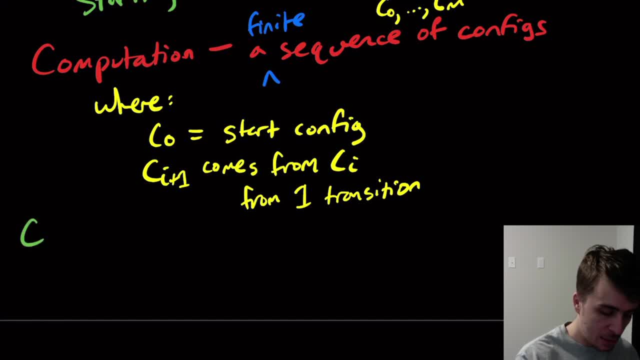 though. So we say that ci plus one- there's a more specific term- is yielded from. so that's the technical term from ci. You can also say ci yields ci plus one. that's also equivalent If applying one transition gets ci plus one. So it's just a more technical term and we're going to be using yields. quite a. 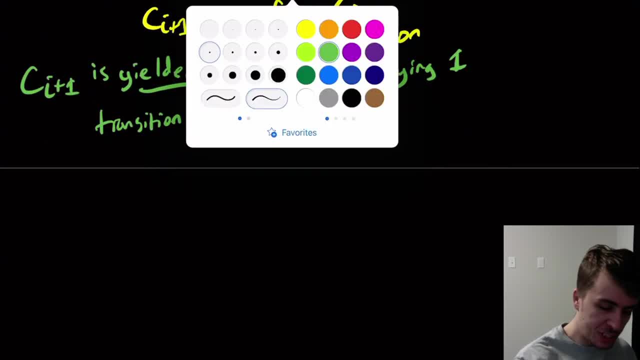 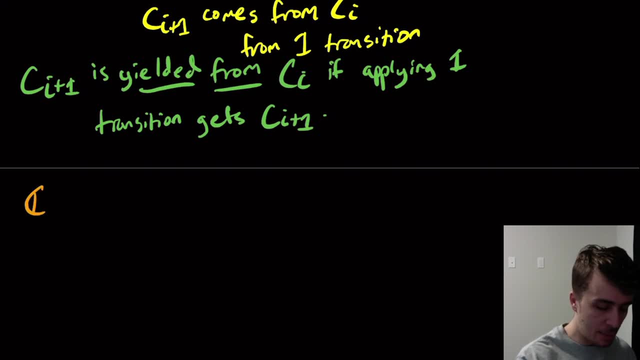 bit Okay. so we're going to say several things that let's call c and I'm going to put a little vertical bar right there to be a computation. Let's say, with configurations c zero through c m, then we will say that c, this computation is accepting. 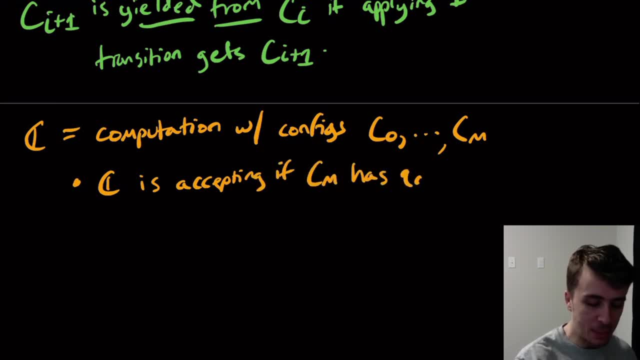 if c m has q accept in it, We will also say that c is rejecting if c m has q reject. and it's impossible, of course, for any configuration to have two states, because it's defined to have only one state And it turns out that we need a third one here, which is that it's 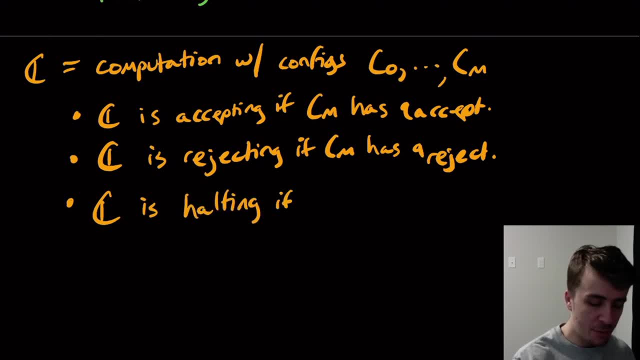 halting, So it's halting, if either accepting or rejecting. Because there are some situations where we can't reason about whether the Turing machine actually stops. So it may be important to say, oh, I don't care what it does, as long as it stops, That's what I care about. So we will say that it's. 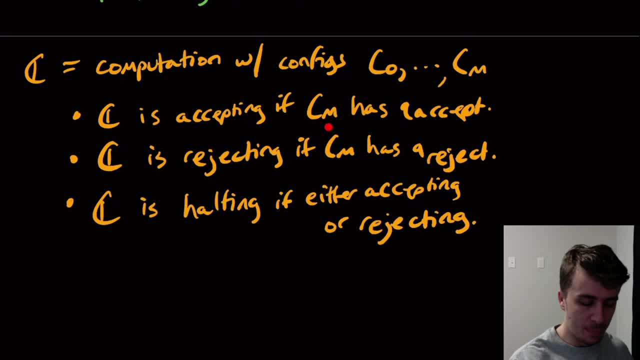 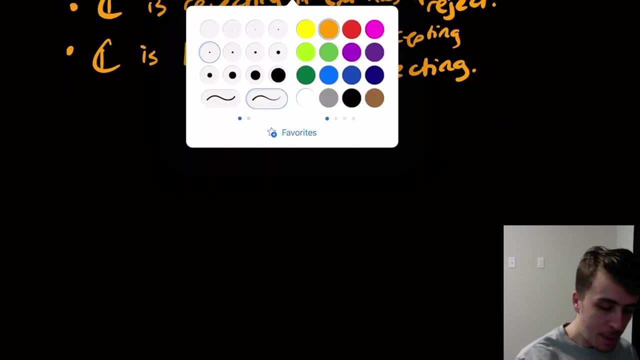 halting if the very last configurer, if it stops at some point, if this is a finance sequence, then it's halting. And the last one has either the accept state or the reject state. Okay, Well, what about the language of acceptance? 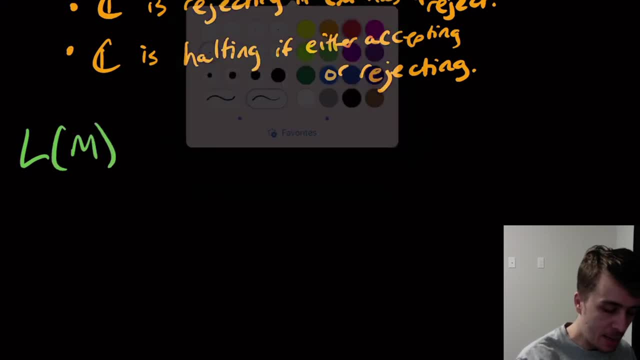 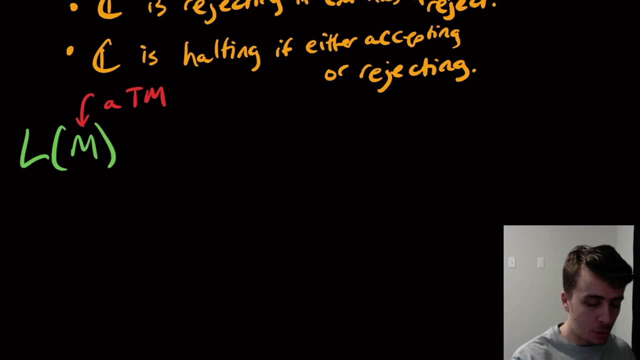 So let's say we want to have a Turing machine, So let's have M here be a Turing machine. I'm going to abbreviate that as TM. So L of M is going to be all the strings in sigma star. Note, not gamma star, because sigma, remember, is the input. 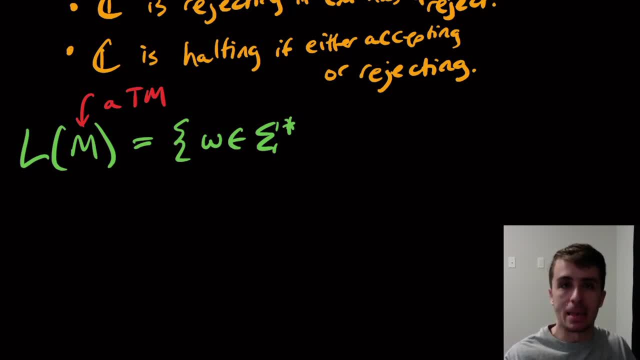 alphabet. The gamma is just the tape alphabet. what goes on the tape? We're only focusing on the strings in sigma star. We never worry about strings in gamma star presented as input. So it's all the strings in sigma star, such that M has an. 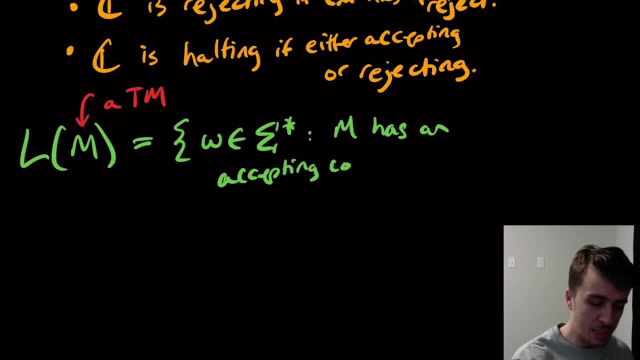 accepting computation on W. So if you run the Turing machine on input W, you will have an accepting computation. so, according to the definition above, So like the example we did before, that Turing machine accepted zero, zero, zero, zero for zeros, And so the language of that machine must have the string for: 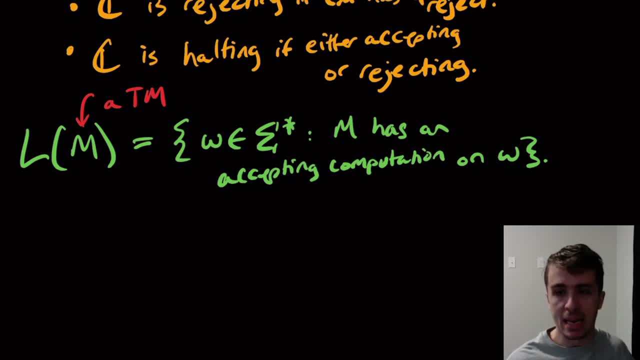 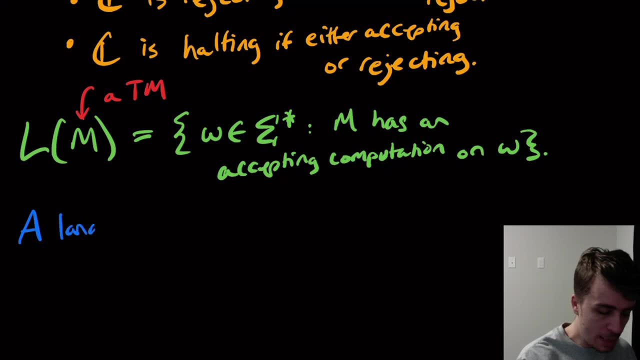 zeros, Just so. it's very similar to a DFA or a PDA or anything. We will say a, so we'll say a language called L is, and the term here is recognizable, so it's recognizable, if some actually I'll just go ahead and do this. 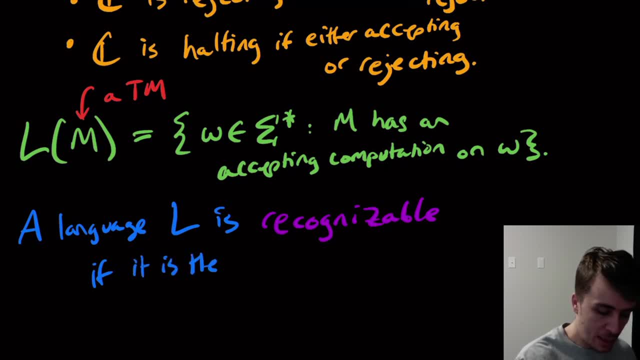 I should write it this way: If it is the language of some Turing machine, M, So if it has some language, sorry, if some Turing machine has that language that you're interested in, it is recognizable. But one thing that we'll note here is: 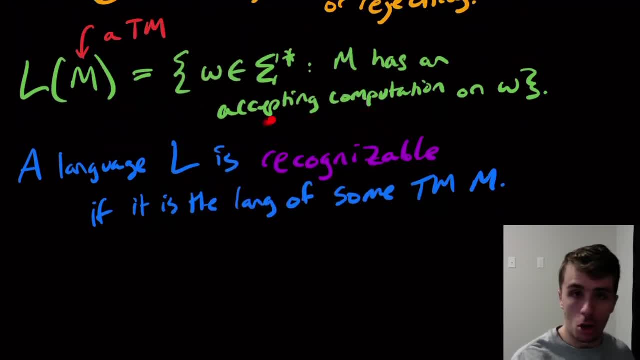 this is not requiring us to halt. So remember that a Turing machine could run forever. So this is just saying that on the strings where it has an accepting computation, it must. it obviously must stop, because computations are finite in length. So here this is. 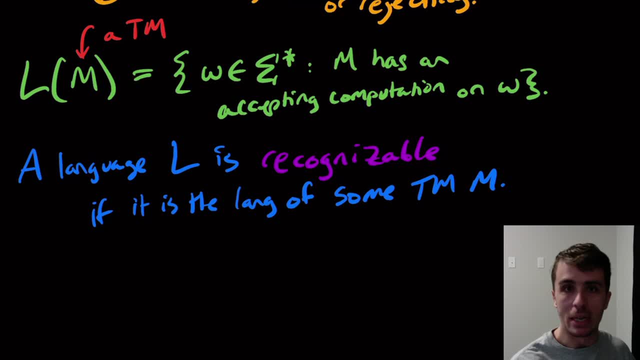 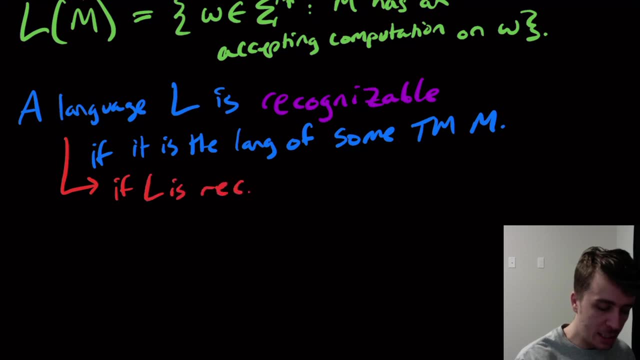 saying that on the strings in the language we're required to halt. So I should say here that if L is recognizable, the Turing machine is only- oops, only- required to halt on the strings W that are in the language. It's not. 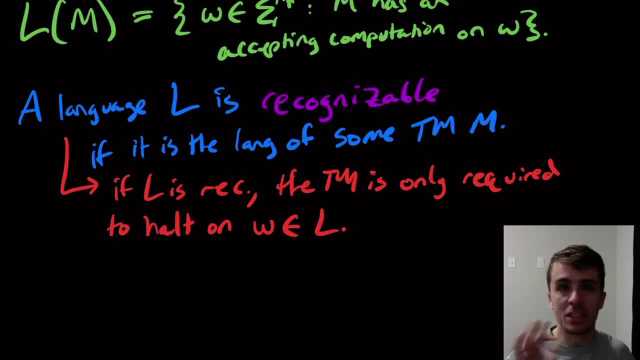 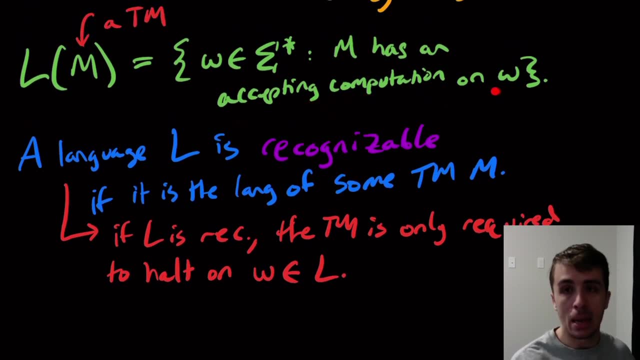 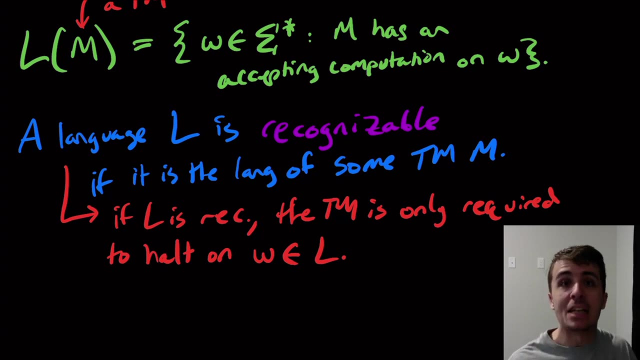 required to halt on the strings that are not in the language. It's not ever required to do that because the only qualification of being in the language is that it stops on that input string, Whereas a DFA, for example, it has to halt on every single input string. In fact, you can modify a PDA, for example, to: 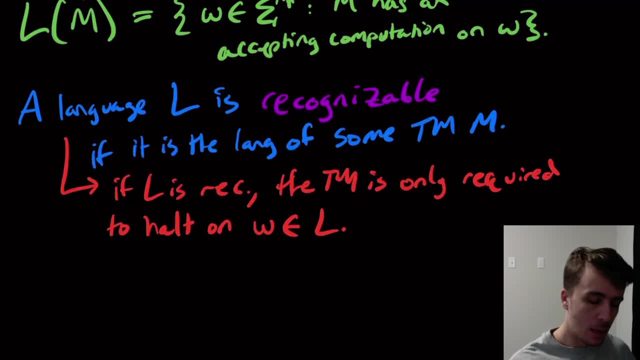 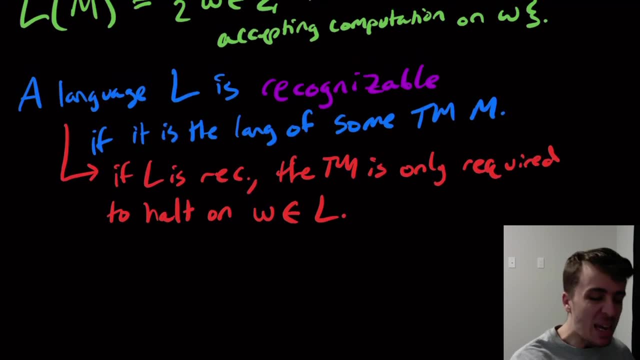 always halt, but that's for a different video. A Turing machine might not halt and it turns out. it's not possible to always require it to do so, But if we have a Turing machine that does always halt, then we can give a different. 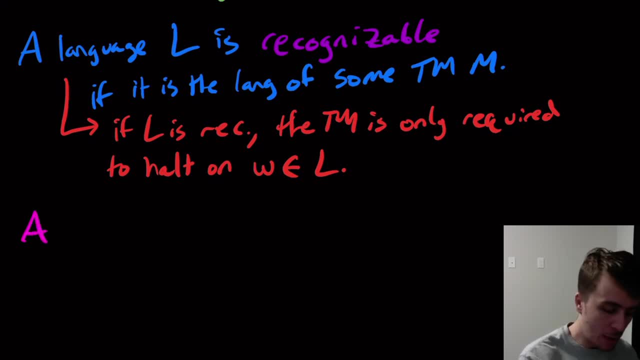 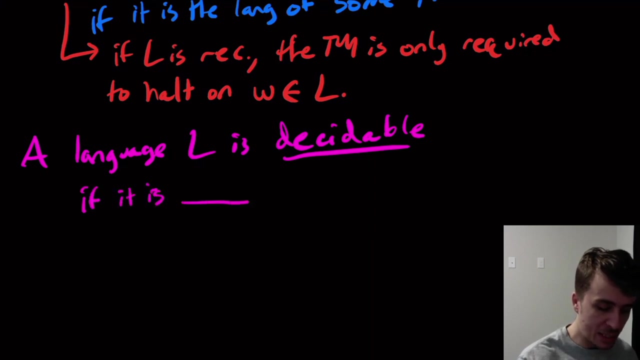 classification to the language itself. So a language L is a decidable, so decidable. or sometimes people put Turing recognizable and Turing decidable. I'm just gonna say decidable because it's easier. It's decidable if it is the language of some Turing machine. M and M halts on all. 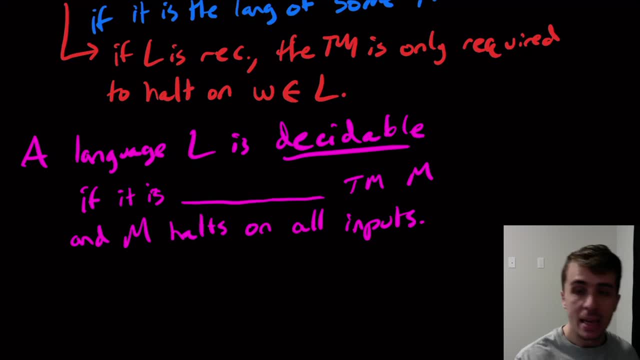 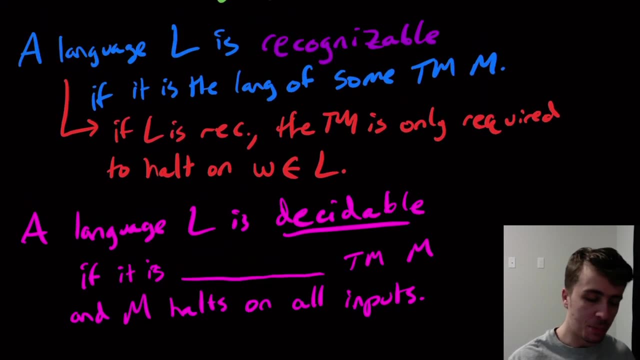 inputs. So that means that it will eventually stop on every single input it's ever given Okay, whereas the one for recognizable- you're only required to halt on the strings in the language. For the ones that are not in the language, it doesn't have to stop. It could stop, but 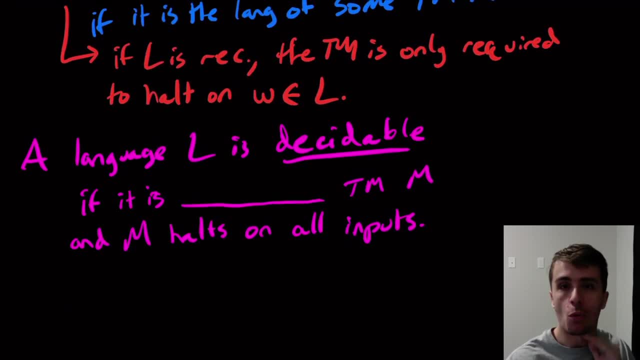 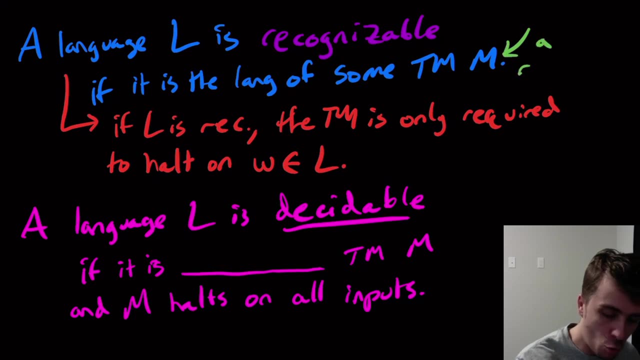 it doesn't have to stop, Whereas for the decidable one, then it's required to stop. So in the top case we're gonna call M a recognizer. So So M is a recognizer for this language And, as you might expect, the machine down here is called a decider. 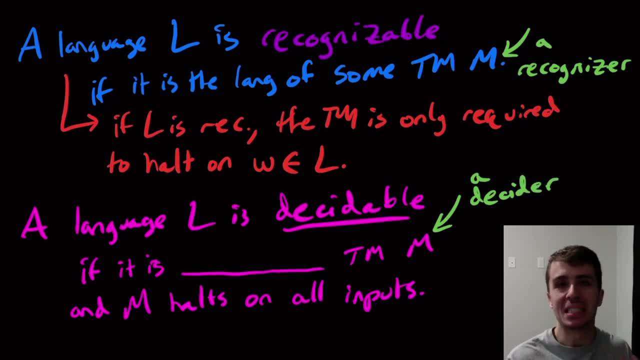 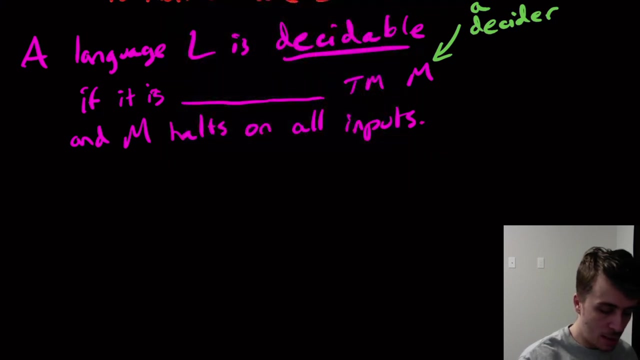 So then we may ask questions about whether there exists a decider for a language or a recognizer for a language. That corresponds to obviously decidable and recognizable, And one thing that you should note here is that if a language L is decidable, it is recognizable, right. 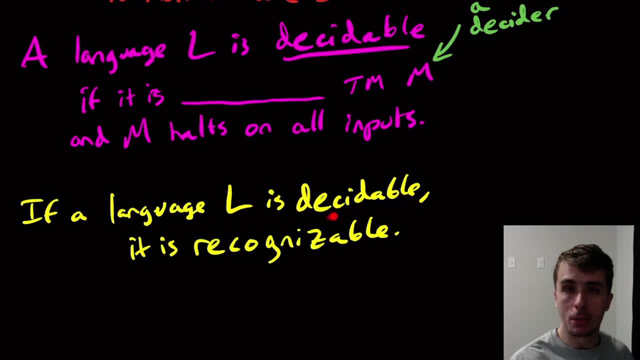 Because if it's decidable, that means that there's a Turing machine that always halts on everything, But recognizable you're only required to halt It's not recognizable on the strings in the language. So the decider for this language, the language here, already satisfies the requirement for being recognizable, a recognizer.